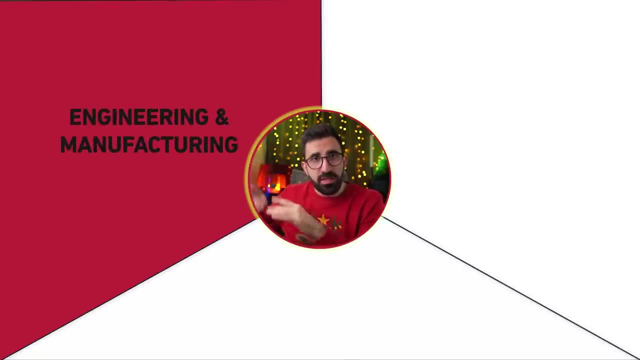 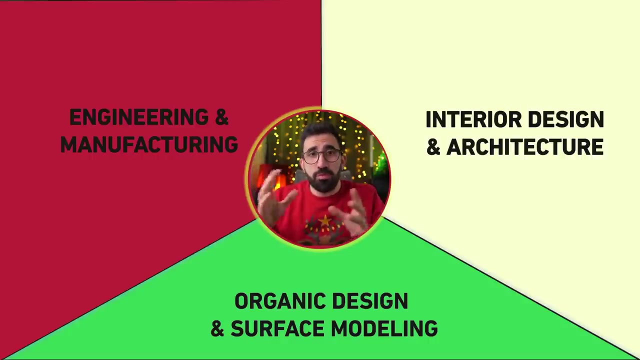 three categories and on this section we have engineering. I will expand each category in a bit. Engineering and manufacturing: Over here we have organic design and surface modeling and we have here interior design and architecture. and before I go to the details of each of these categories, a lot of you might have come here for 3D printing. Let me just get. 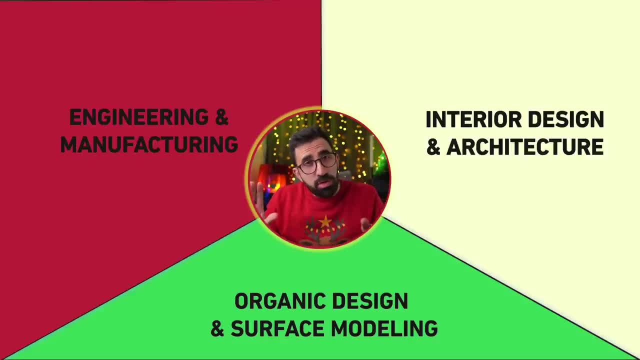 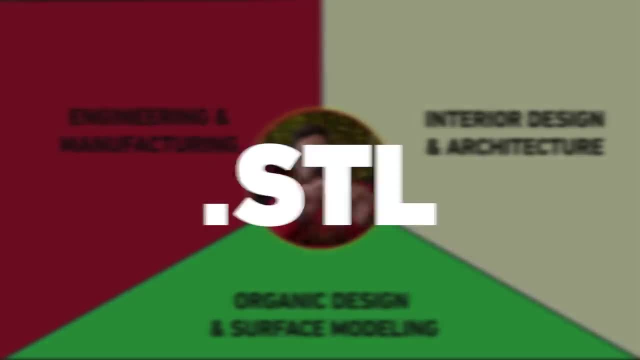 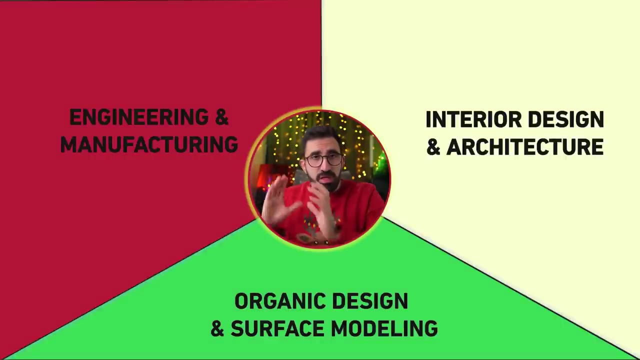 this out of the way: regardless of which of these categories you're going to fit into, which industry you are in, you can still 3D print your model. okay. 3D printers only require STL format, and almost every cat out there can generate STL, so this is not a category. okay, Focus on the industry you're 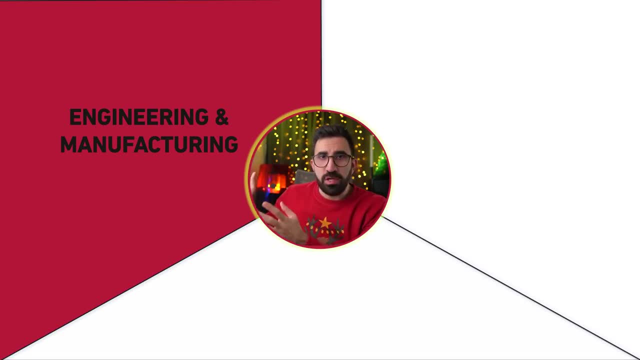 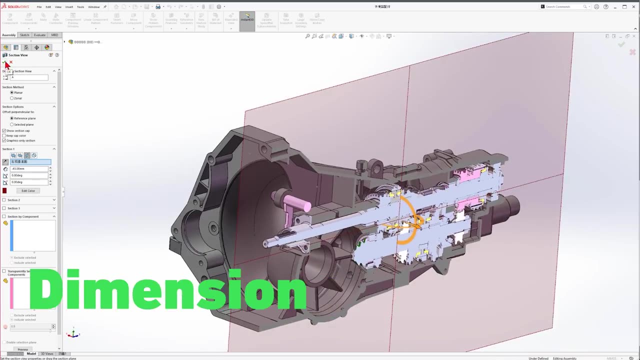 in Engineering: organic design and architecture Engineering. what do I mean by that? If you want your components to be accurate, if you want it to be fabricated, manufactured, fit together. the dimensions and tolerances are important. surface finish is important. for you, these are under. 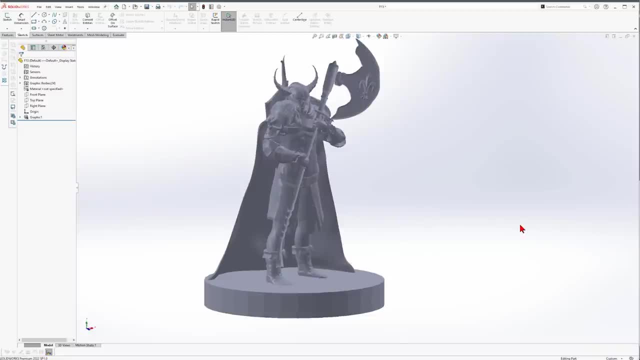 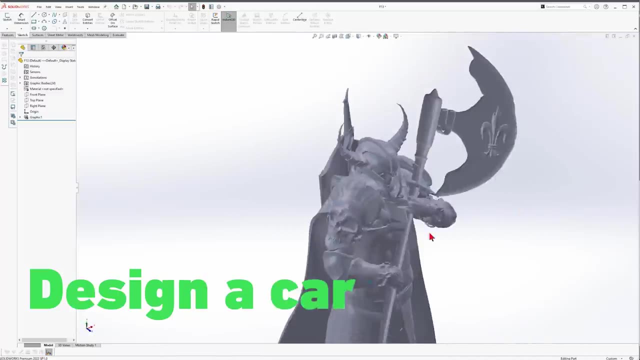 engineering, Organic design and surface modeling. If you are in the gaming industry, if you want to create a character, if you want to design a car, something that has an organic geometry, like a skull of a human being, like a bone, this is the industry you want to look at. keep that in mind. 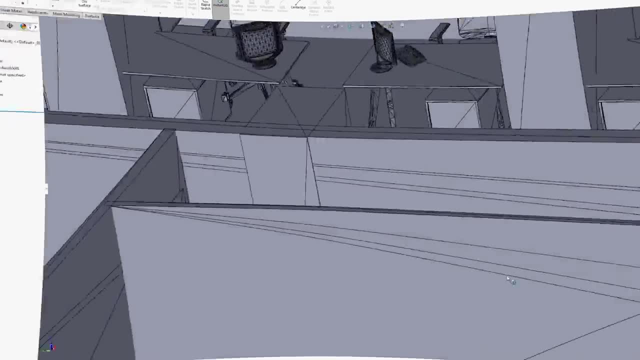 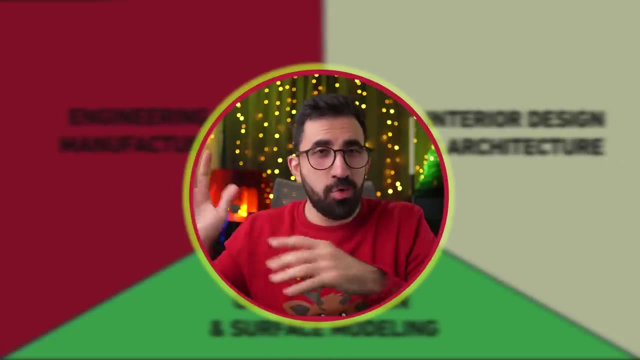 Interior design and architecture. it just goes without saying what that is okay. No one- and I mean no one- is an expert in all these three categories. usually people are expert in one or one or two. I am expert by category in engineering and not the other two, so I'm. 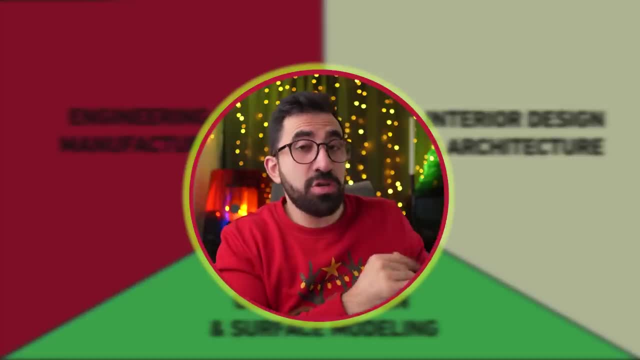 going to brush past these two- that is, organic design and architecture- much faster. get it out of the way and send you on your way to do your own due diligence on other videos. Unfortunately I'm not an expert. I don't want to just name drop bunches cat out there. oh, there's blender there. 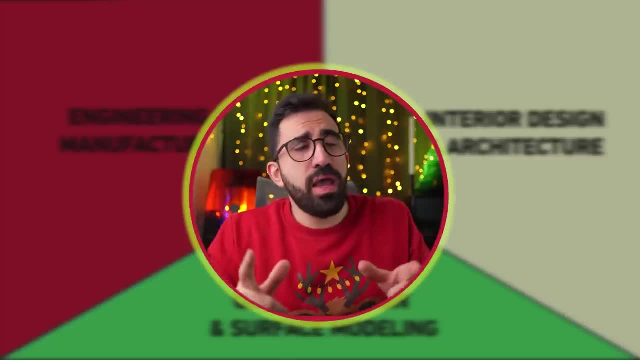 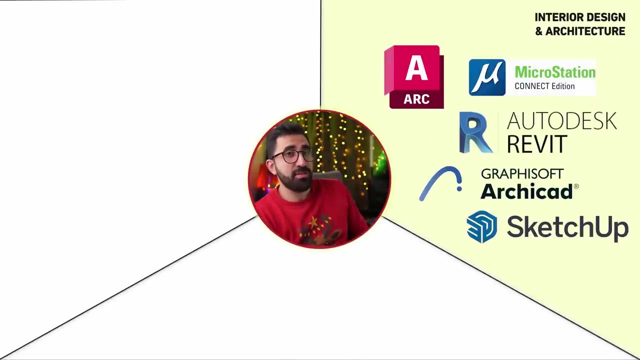 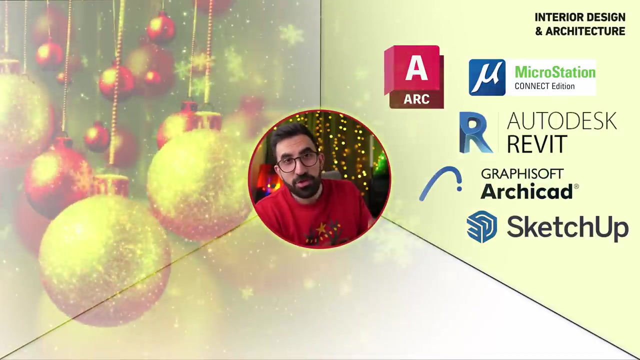 is this and that that doesn't do you any good. There are software that can cover both, like blender- I know blender is a god tier- or 3ds max, and there are software that are specifically for one. for example, if you're an architect, if you want to design a building or an interior design, these are the cat that you should be looking into. since I am not experienced with them, I don't want to comment on any of them. okay, but just keep that in mind. this is as narrow as I can make it for you right now. unfortunately, if this is you and if you have to leave this video at this point, I wish you merry christmas and happy holidays. 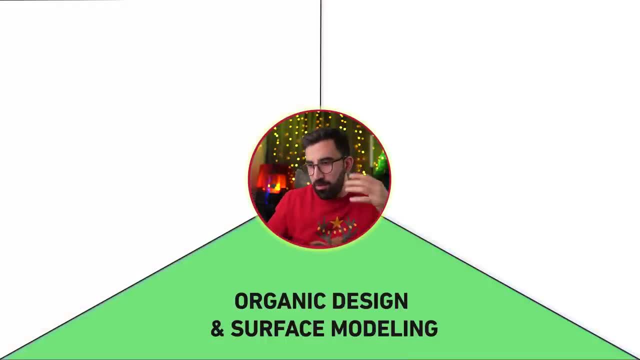 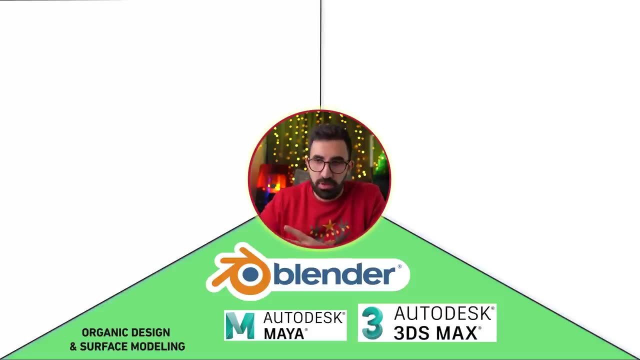 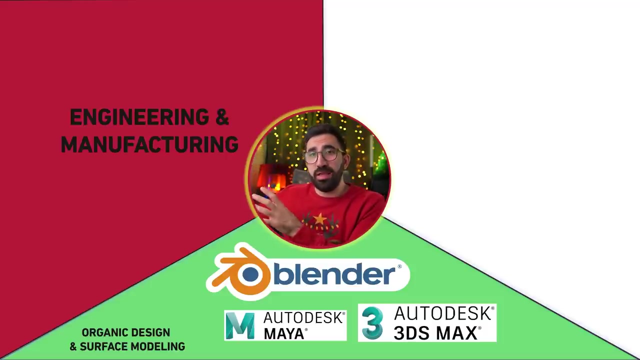 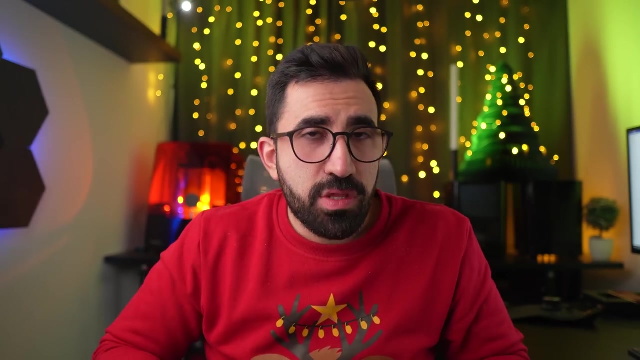 Similarly, for the other people who want to do organic design, like character, or you want to do artsy stuff- blender, maya, 3ds max and a lot more- you're going to look in this direction. okay, you guys, stick with me for a second, because I have something that used to belong to the engineering category and now it has expanded into this and I know a little bit more about that one that can help you. they happen to be the sponsor of this video as well. you know I'm a solidworks guy, but I'm not talking about solidworks per se. it's solidworks cloud offer, which runs. 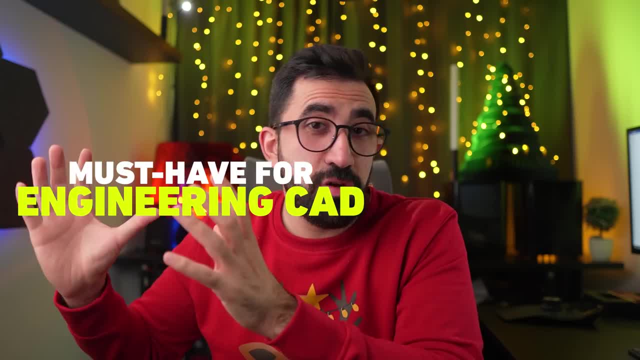 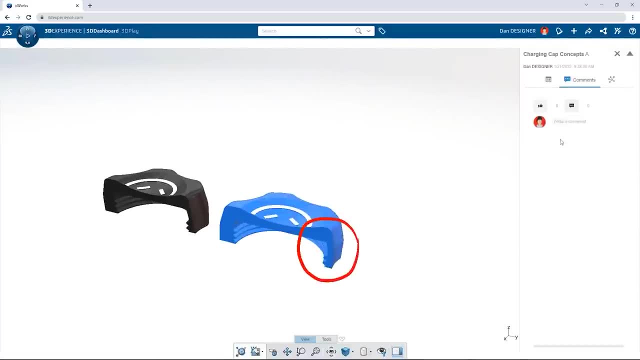 on the browser. it has all the features that an engineering cat must have, like dimensions, accuracy, tolerancing and everything. also, it offers you the sculptor tool, something that works with polygons like blender, that you can form and drag into whatever shape that you want and create organic. 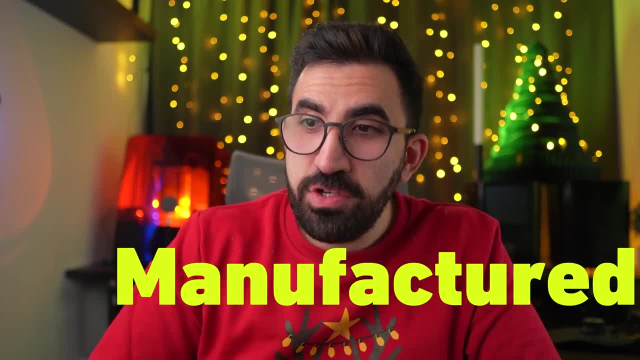 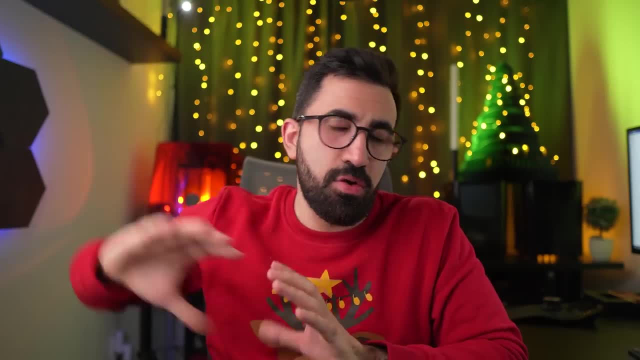 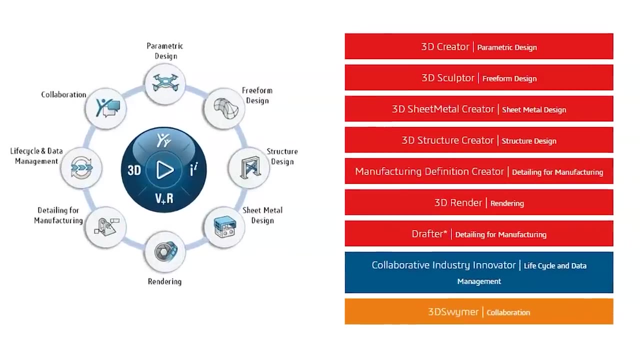 geometries as well, but organic geometries that can be manufactured, that are accurate and reliable and are based on dimensions. new solutions like this are a bridge between these two categories, so the solidworks cloud offer combines proven design and collaboration tools that allow all your stakeholders to work together from anywhere, on any device, using 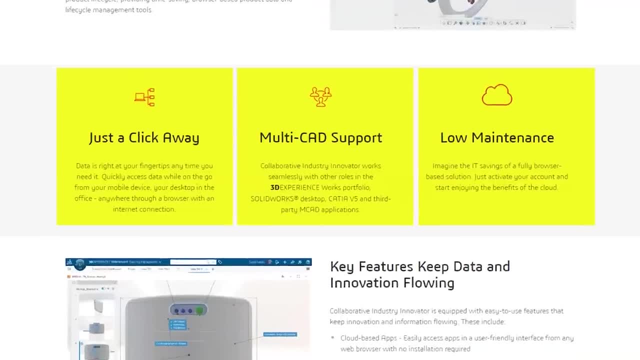 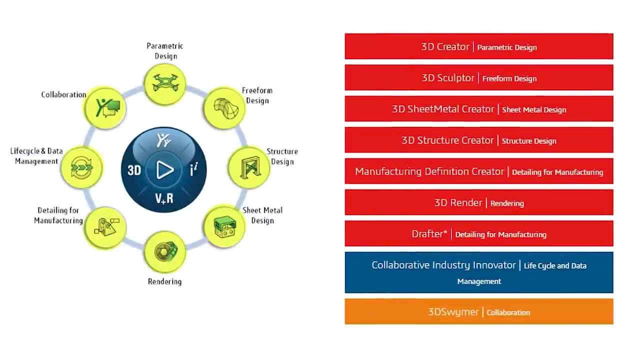 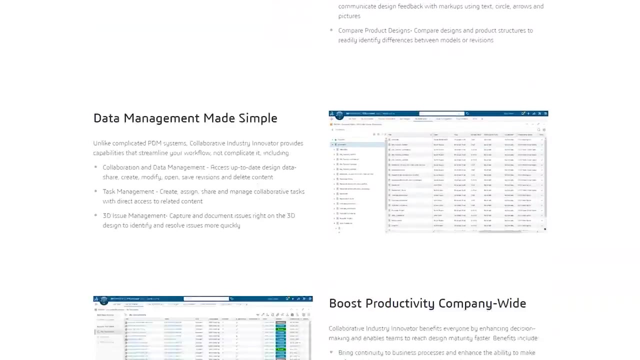 browsers. you don't have any costly IT overhead because it's cloud-based, and you can scale easily as your company grows. the solidworks cloud offer also includes designing, collaborating and reviewing from anywhere between teams. it is a single modeling environment for parts and assemblies and it allows you to focus on your design, so there is no need to worry about organizing. 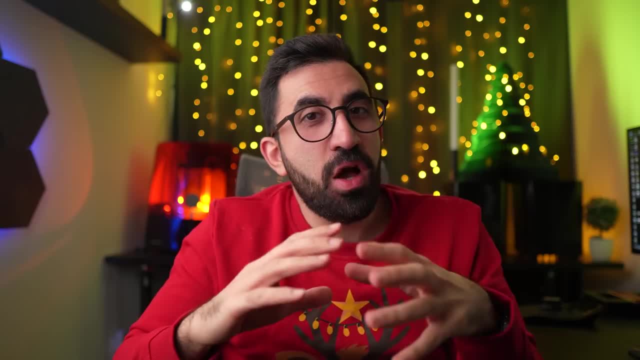 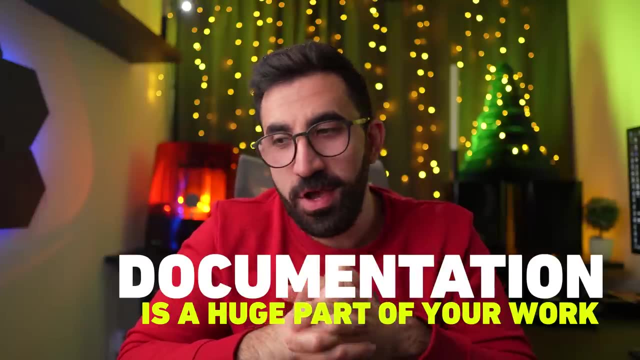 your files, because when you actually get a job in a company, your job will not be limited to only working with the cat. the documentation is a huge part of your work. whether you want it or not, you're gonna have to keep your file organized, and a cloud-based cat like cloud. 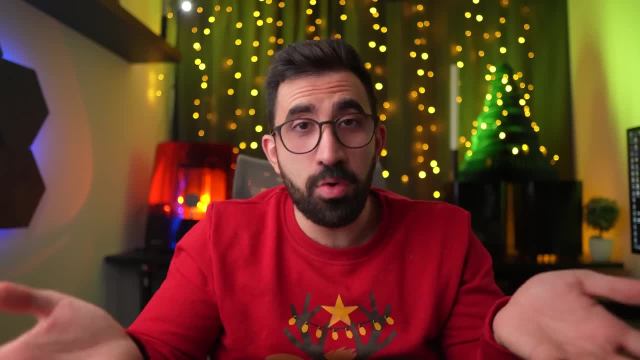 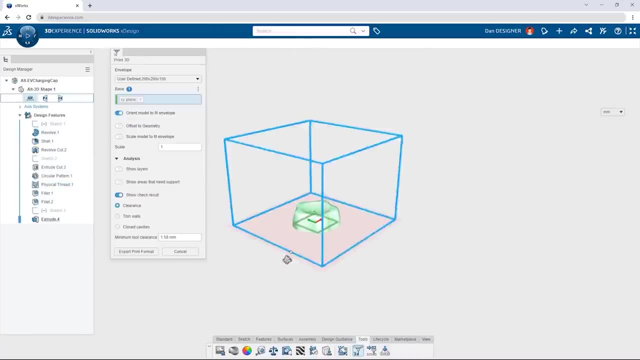 offer from solidworks does that for you automated and it cannot go wrong. that's a very huge plus point on that. also, there are some new and intuitive features compared to solidworks desktop version, which allow you to change design intent without the rework that's required with the you know. 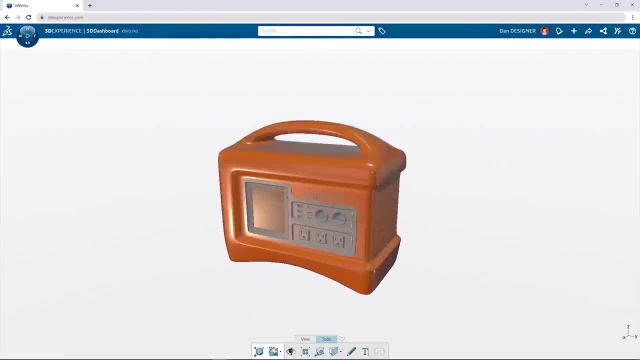 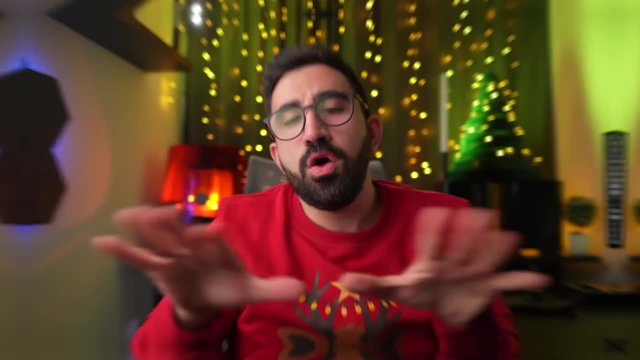 the stop version, the parametric modeling- you can always be connected to the cloud-based cloud offer to your members in your team and comment on each other's work, ask for help, get access to your content from different locations. also, it doesn't need any maintenance because the desktop version sometimes 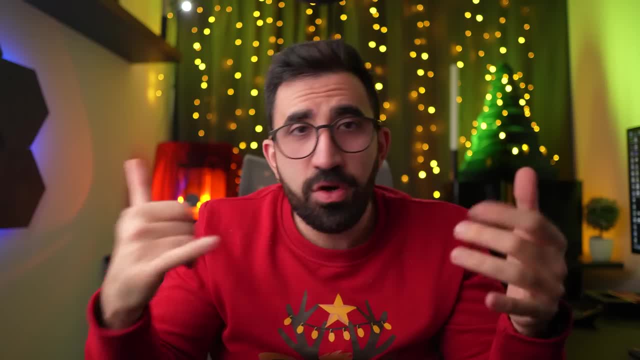 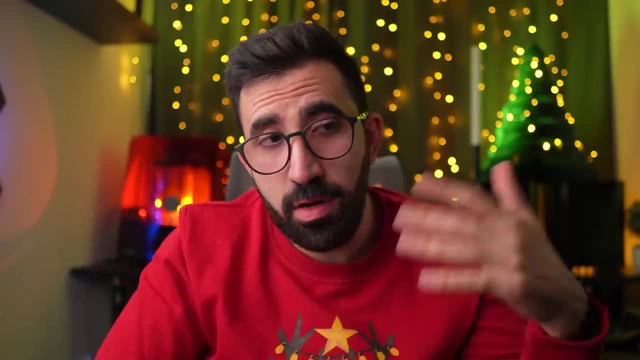 because it's on your local pc. if it gets stuck, it gets stuck. you're gonna have to call the support to help you. but this one runs on the 3d experience platform and it doesn't need any backup or maintenance. everything is there. it doesn't get stuck and if it does, before you get to know it. 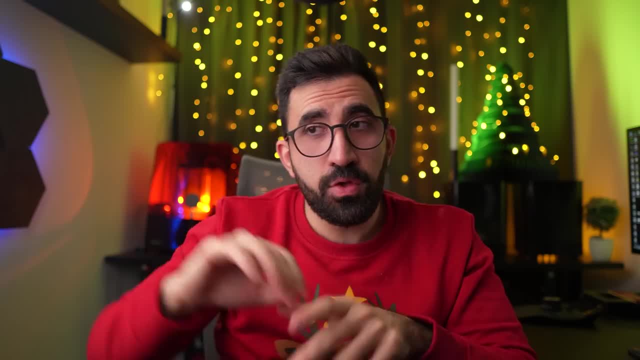 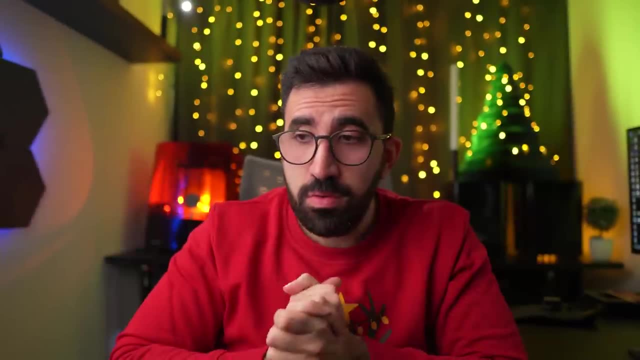 they have solved it already. this is a huge advantage if you want to work with a cat, and also organic design on the cloud server, which is new, okay. so yeah, they are the sponsor of this video, by the way. solidworks cloud offer. i'm gonna put the link to that in. 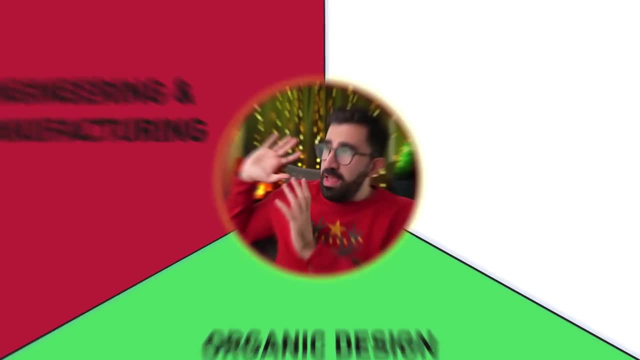 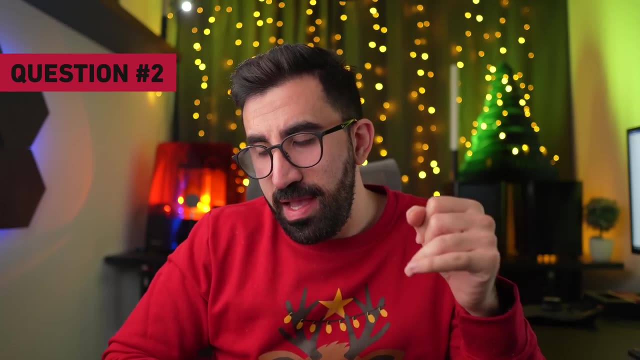 my description below. it's actually salvagecom, forward slash cloud, and if you want to go to engineering these two, you guys, engineering and organic design- you're still with me. next question that i'm gonna throw at you is that desktop or cloud-based? so there are two different categories. 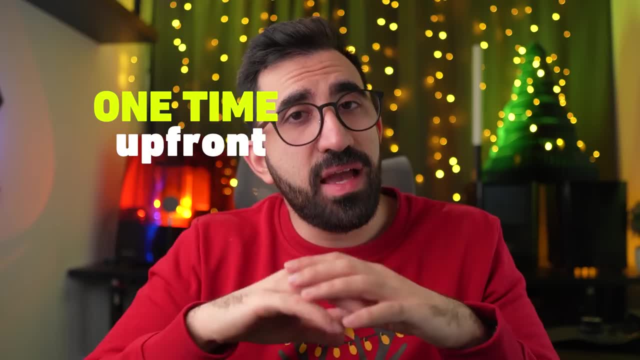 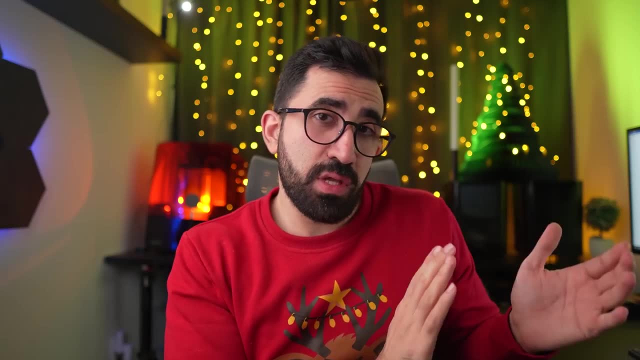 of cat right now, the ones that you pay one time up front and you get it permanently and you install it on your pc. it's called a desktop version, something like solar works, and it has its own pros and cons which i will get into in a second. and there is this new. 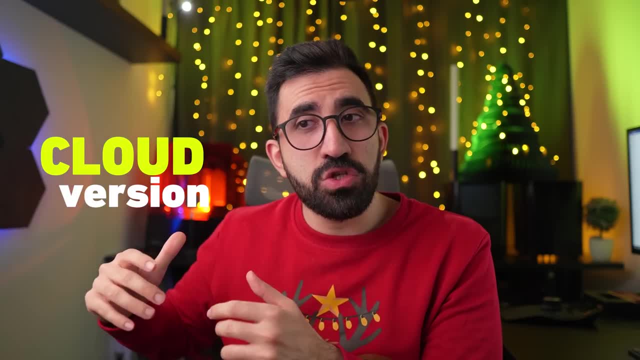 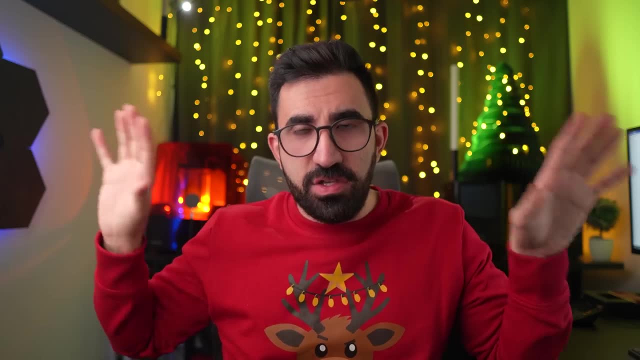 version that has been around for a couple of years now- cloud-based, which you pay on a monthly basis. usually there is no big upfront fee like the desktop version. you run it on your browser. advantages and disadvantages. the cloud-based is cheaper to start if you're a small company- small. 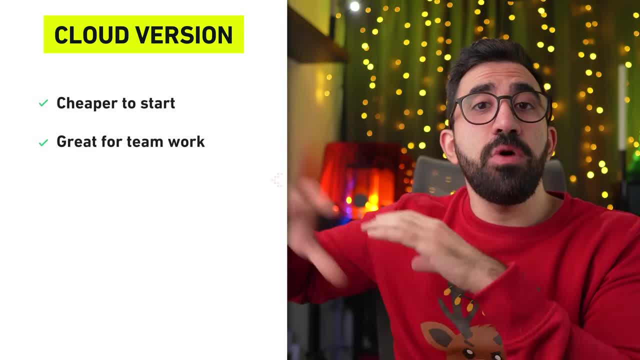 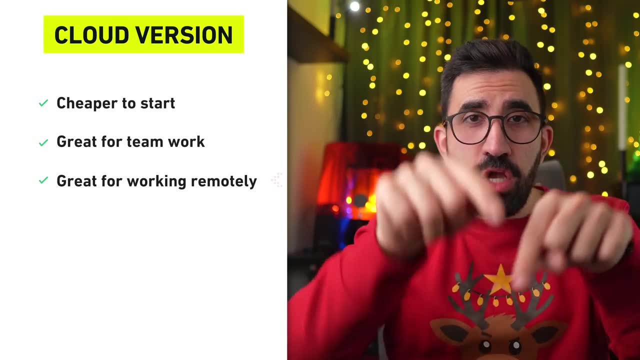 business is great for teamwork, when you want to share your file among your team or if you travel a lot. if you don't want to be dependent on one local computer where every team member has to log into and work with that, okay, everybody can access that from wherever they are, as long as 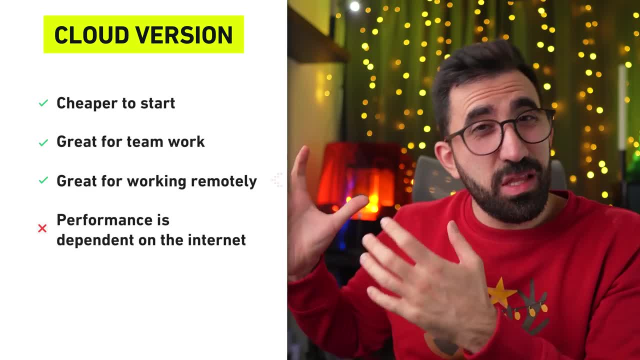 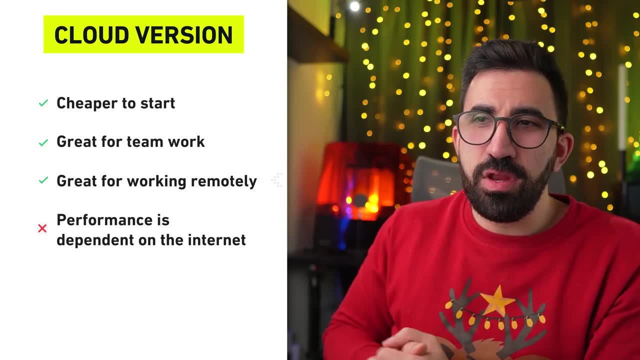 they have internet connection. the disadvantage of that is sometimes it's a little bit laggy, it's dependent on internet. if your internet is not good or the part becomes too heavy and your computer cache is not supportive, so it can become a little bit slow. but if you are, for example, ahead of a different company. you can access that and download your version computer to see what's in it and then take a look at how they're actually weil and check thatлинq. what are the correct settings about? and? or you're a shop owner and you have people. 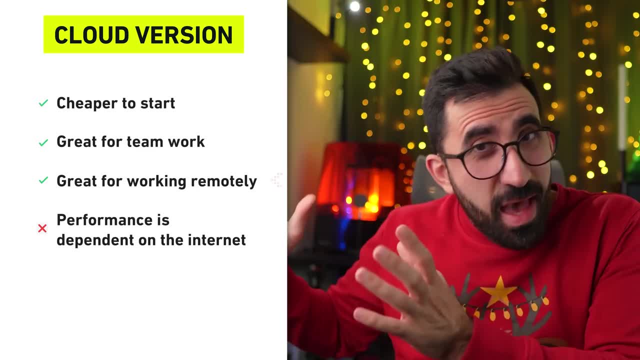 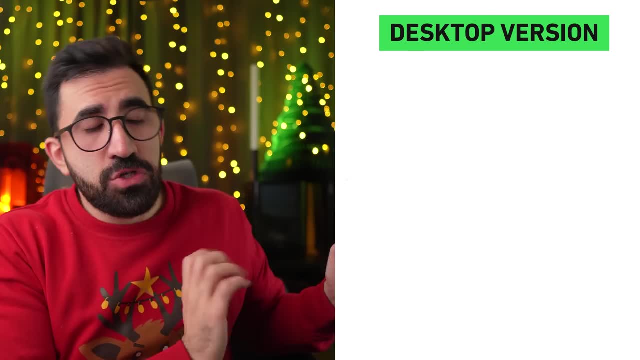 two, three, four, five or more working under you. you might wanna consider that. Look into softwares like Onshape Fusion 360 that are cloud-based. give it a go. The advantage of the desktop version is that you only pay one time. 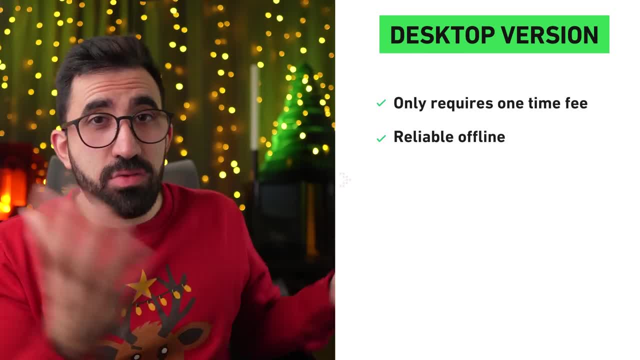 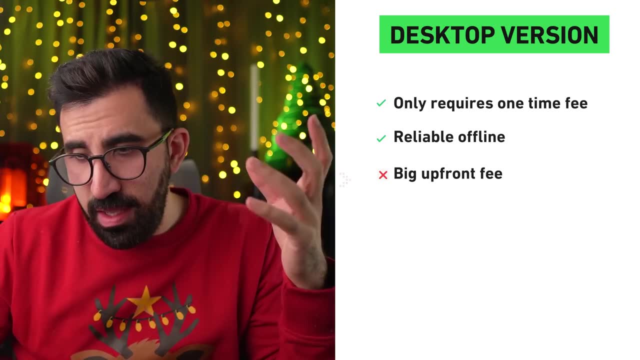 you get all the features unlocked. it doesn't get laggy, it's there, it's reliable. okay, Whether the internet is there or not, whether your browser gets too heavy, it's just there, it works. But there are so many buts- okay. 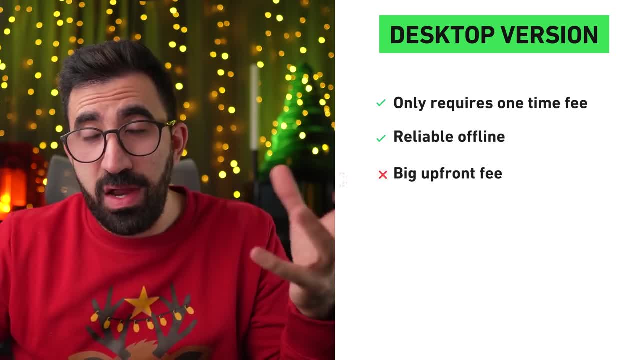 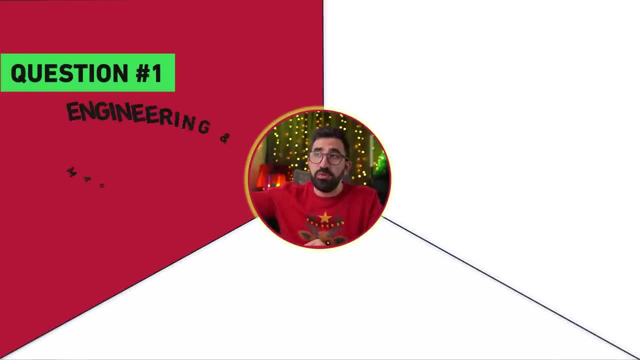 I could talk about this for hours, but nobody would wanna hear me talk for hours. That's why I'm trying to pack as much as information as I can in this short time. Hopefully by now you have decided whether you belong to the engineering category. 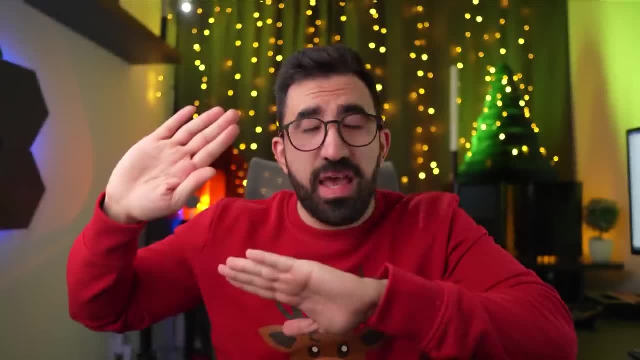 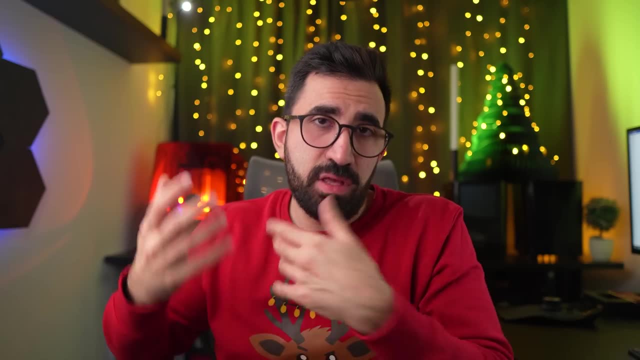 or organic design and surface modeling. okay, Keep these two in mind. And after that I asked you whether you wanna go for cloud or you wanna go for the desktop version. So keep that in mind too. We are narrowing it down, And at the end I will give you a couple of options. 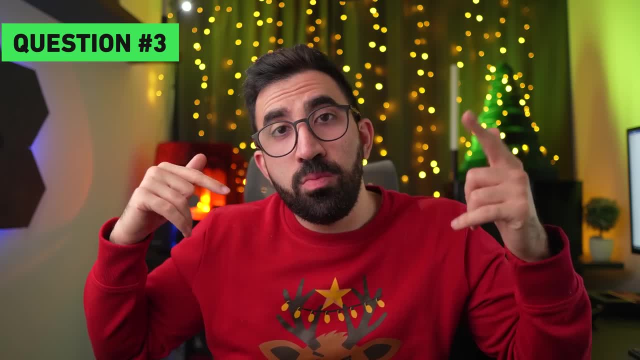 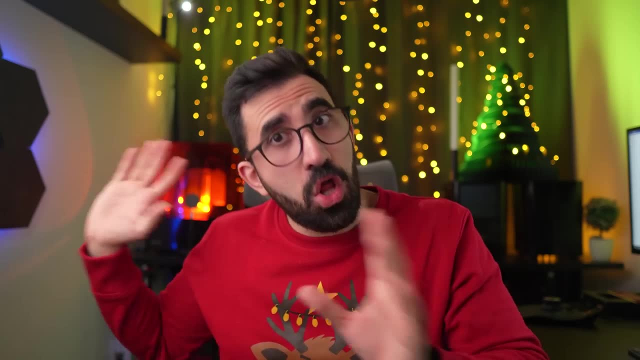 that remain. The third question I wanna throw out to you is that, whether you work more with 2D or 3D, Don't underestimate 2D. I have been working in the hard valve industry and implant stents for a long. 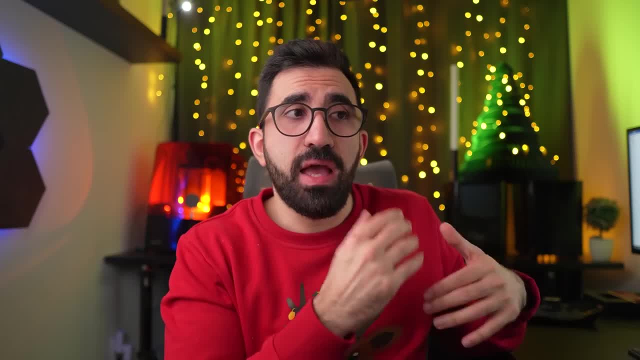 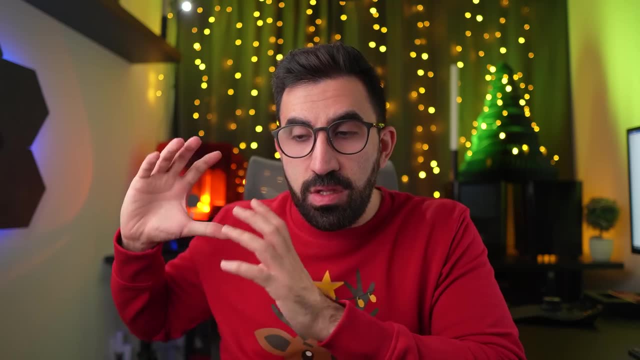 long time. A good portion of my day was spent with 2D. I had to design a lot of entities for the laser path, and 2D was the cat we needed, While software like SOLIDWORKS, Inventor, Fusion 360. 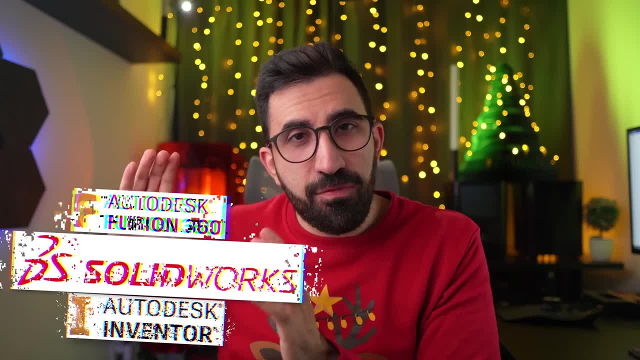 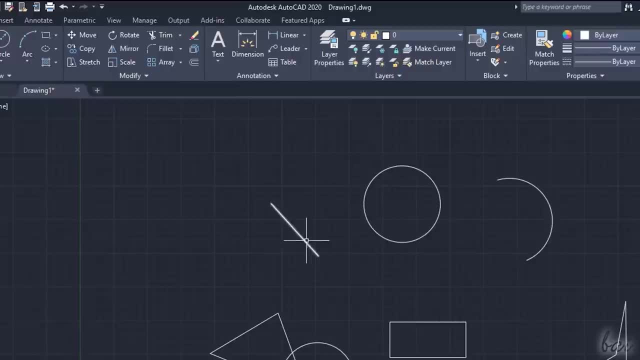 are really good with 3D. when it comes to 2D they slow down and they fail you. They don't have the right tools to handle what you wanna do. 2D- perfectly. What comes to mind? AutoCAD- perfect for 2D. 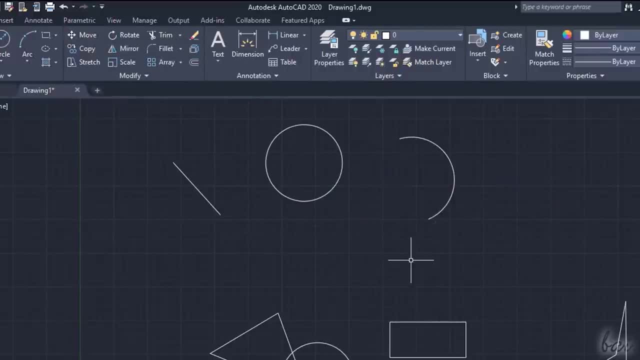 I wanna stay away from it. when it comes to 3D, I mean it's good, but there are better options with better interface. It's a nice and easier process and faster. So for 2D I would go to AutoCAD. 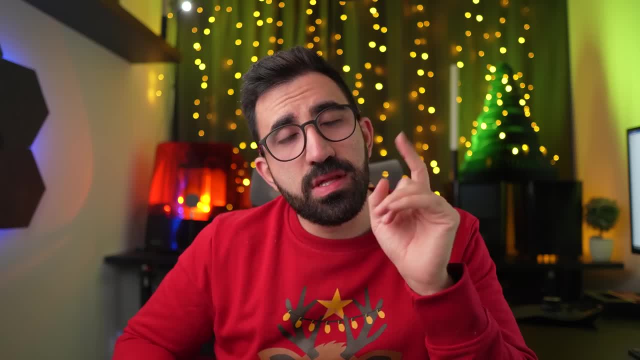 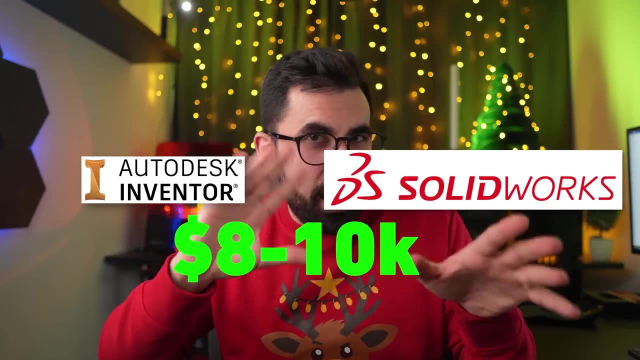 and for 3D, I would go away from it. The next question I wanna ask you is the price. How much you wanna spend Free a software like FreeCAD, medium range like SOLIDWORKS or Inventor- around eight to 10K. 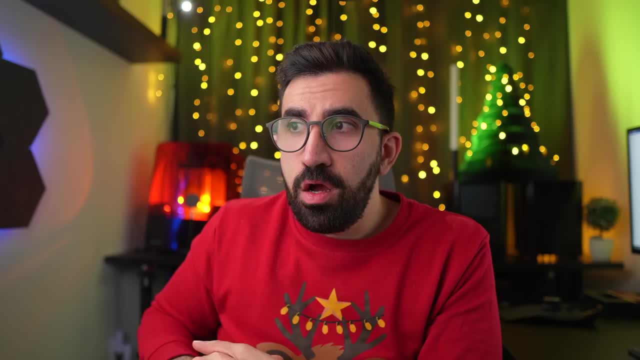 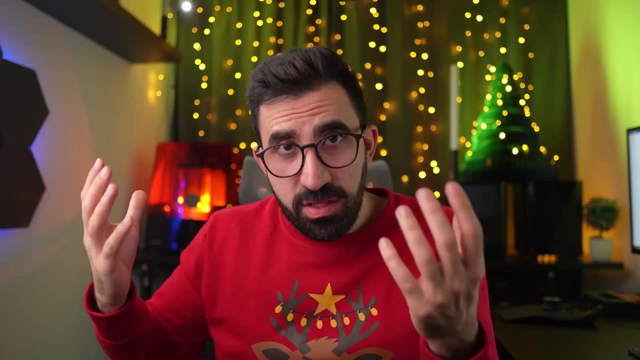 and high tiers like CATIA 100K. You might ask me, Arjan, why would I wanna consider something so expensive when there is a free stuff? Well, obviously, the more you pay, the more you get, Depending on the industry and the business you're in. 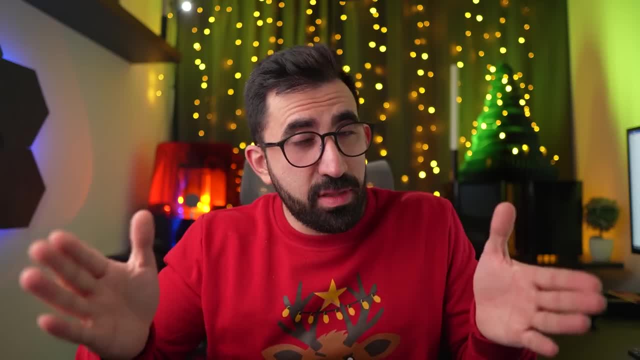 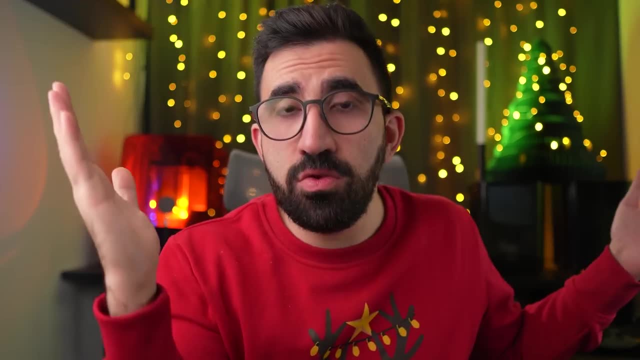 you have some minimum expectation. You should have minimum expectations from the software you buy. So FreeCAD is good for a lot of stuff. For many of you it might be satisfactory. So you don't need to pay anything. But usually free stuff are for non-commercial use. 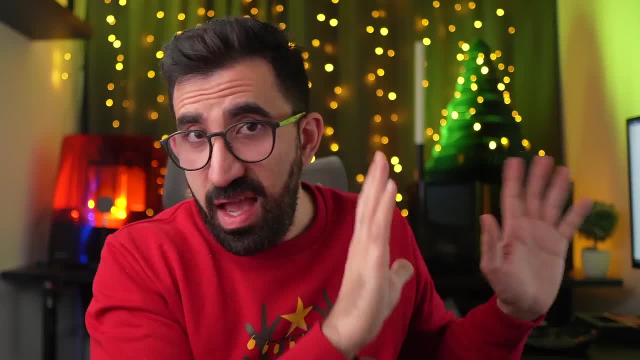 I'm not sure about FreeCAD. Check it out. Make sure you can use it commercially. As long as it does what you need it to do, then it's fine. go for it. Medium range, like Inventor, SOLIDWORKS, AutoCAD. 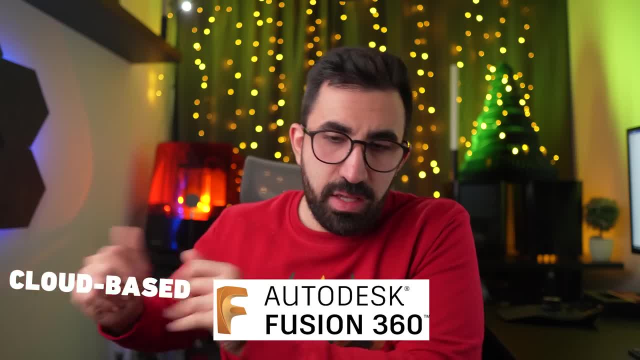 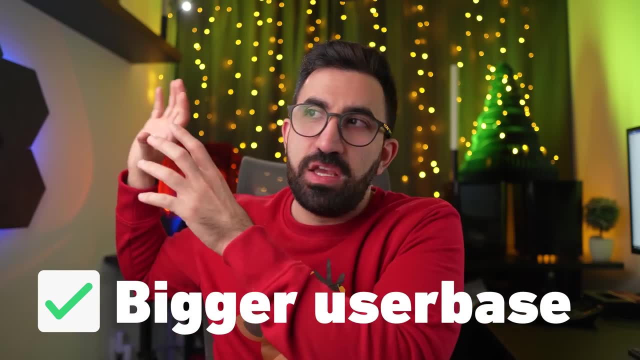 These are desktop versions and Onshape Fusion 360, cloud-based. These are where you wanna be. The user base for these mid-range software is much bigger than software like CATIA NX or Creo, which are high tier. There are smaller targeted niche groups working with them. 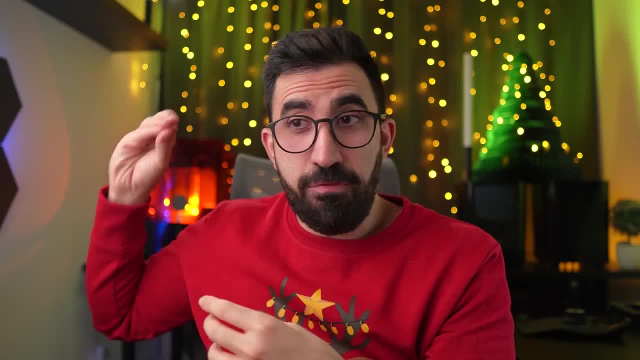 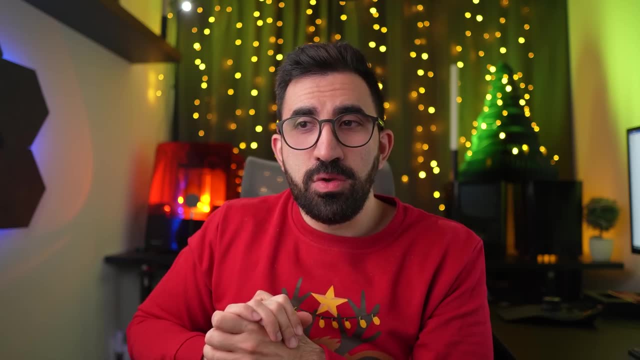 Companies like Boeing. Yes, you would be specialized. Yes, if a company wants a person that is expert in CATIA, your chances are higher because your competition is lower, But on the other hand, when you get stuck or you're looking for a solution on the internet, 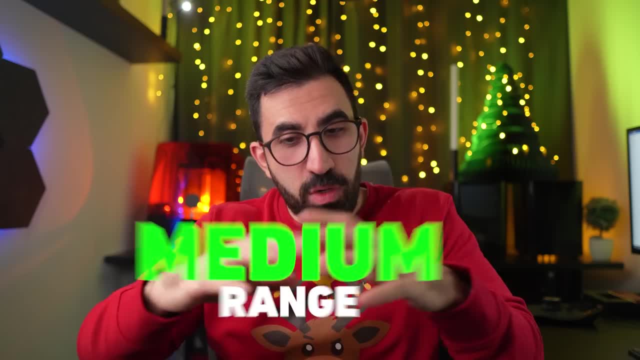 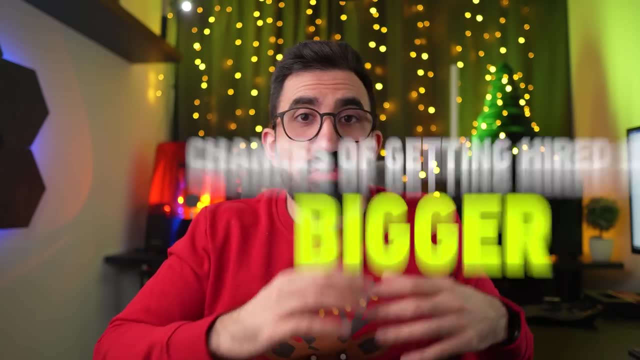 the number of people talking about that problem is also less. But when you come to the mid-range, where SOLIDWORKS and AutoCAD are, the user base are bigger. More and more companies are switching to SOLIDWORKS, for example. your chances of getting hired is bigger. 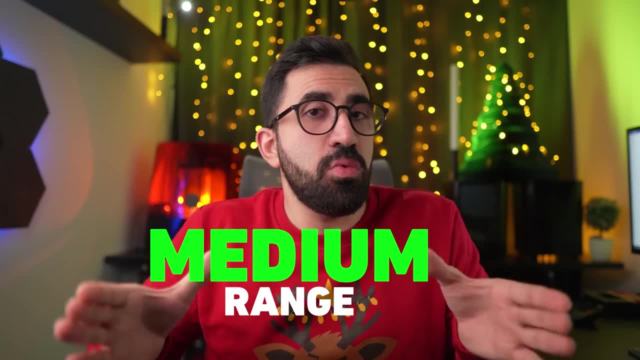 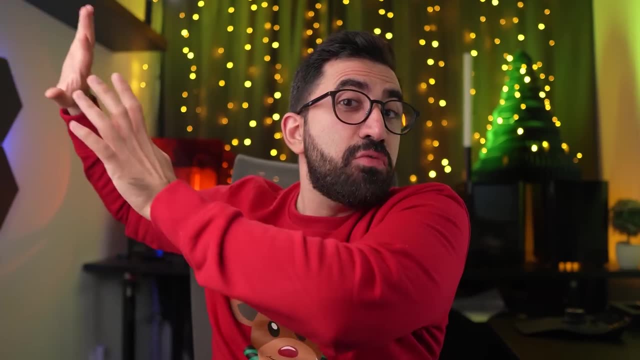 This is where I recommend okay, Because this mid-range does everything you want it to do, Unless you have some specialized use like CAM or hard simulation, manufacturing simulations. yes, you could just move toward the high tier, But for now, stick with me with the software. 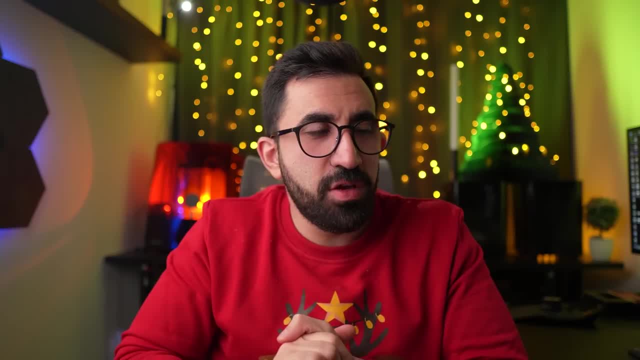 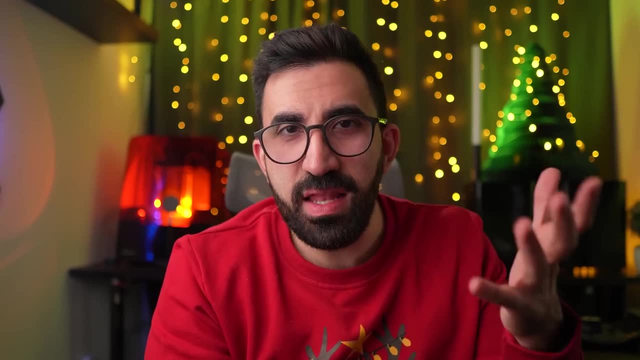 Lastly, I wanted to talk about the price of each of these software, but I realized this video will stay here for a long time on YouTube and the prices are changing all the time, So it will not be valid anymore. I highly suggest you to go to their website. 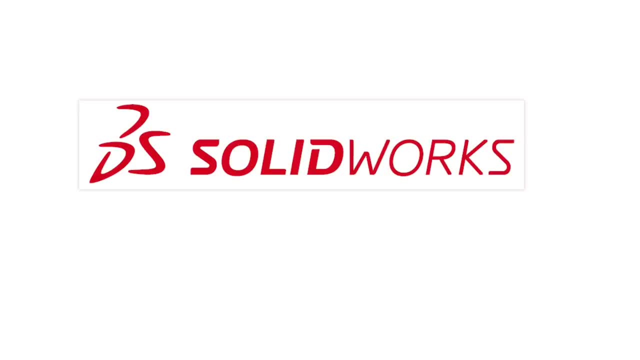 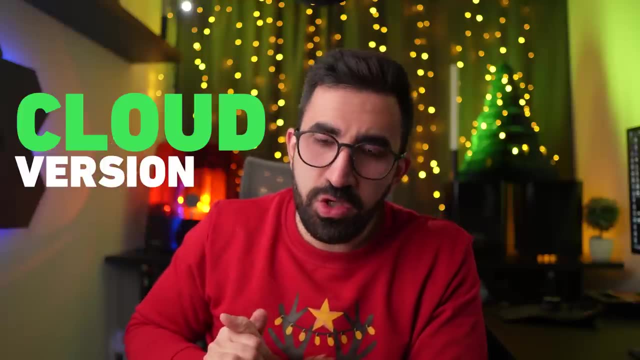 check for their price. For the local software like SOLIDWORKS or Inventor AutoCAD, I told you six to 10K depending on the license you want to get just the range And for the cloud one, usually it's around 1500 per user per year. 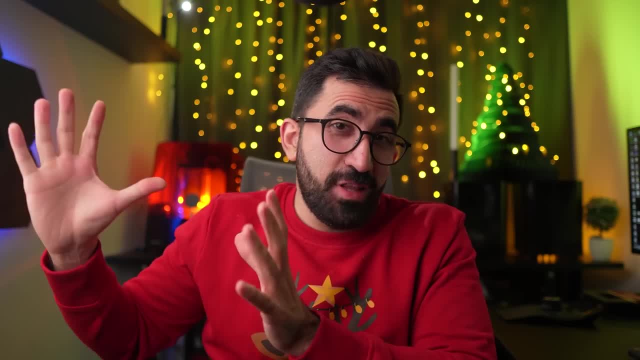 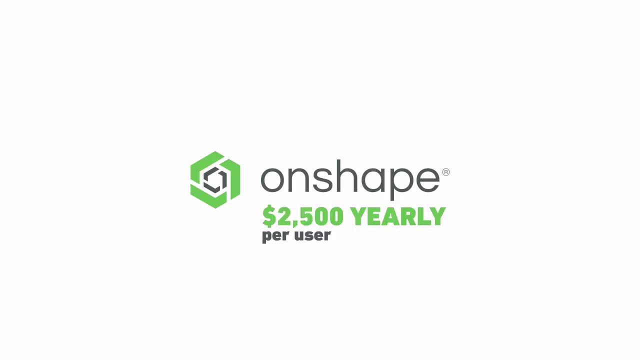 depending on the license, it could go higher. It could get more expensive on cloud, depending on the number of users you want to get. For example, on shape, professional is $2,500 per user per year And if you're like 10, you're you know. 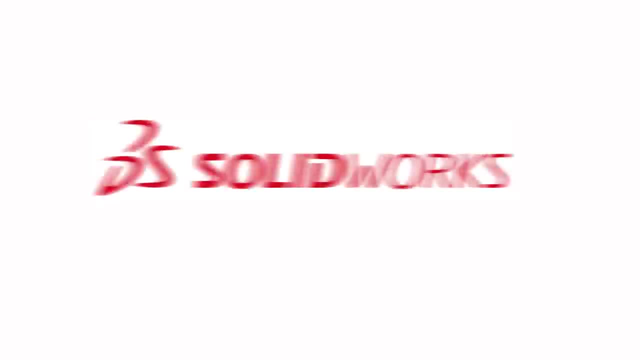 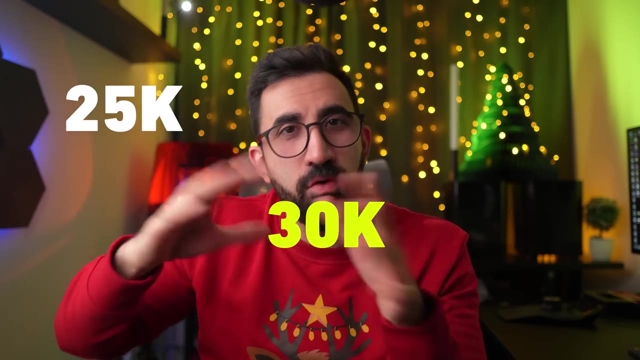 paying 25K per year, While for SOLIDWORKS, if you get three licenses you pay 30K, but it's permanent. Almost 25K for one year, 30K forever. You have to do your math on that. 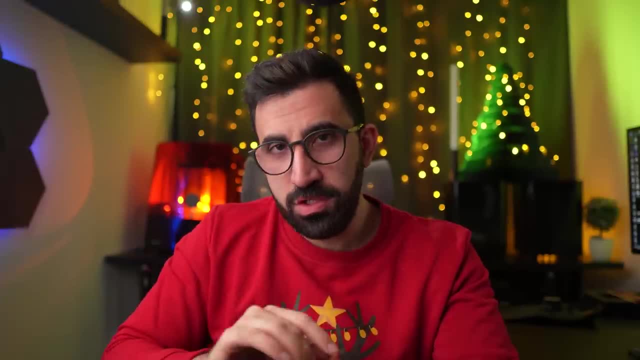 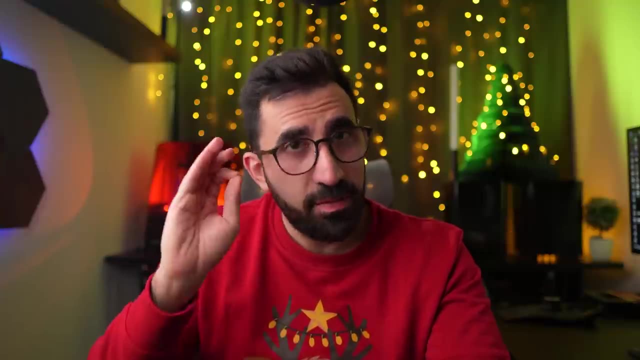 depending on the size of your department or team. If you are still watching to this point, I really thank you for watching my video, So let me throw in one bonus for those of you who are still here, If you want to go for SOLIDWORKS desktop version.